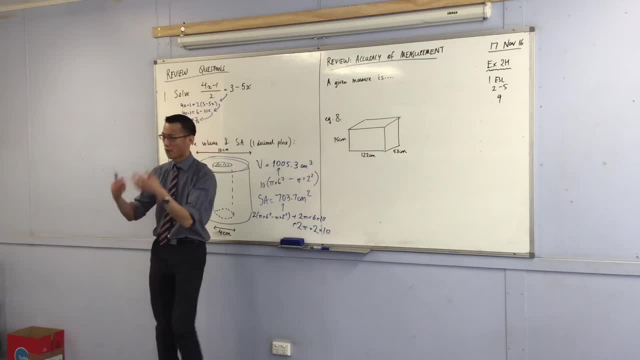 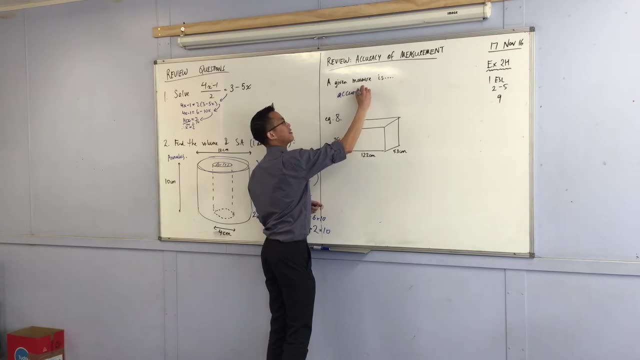 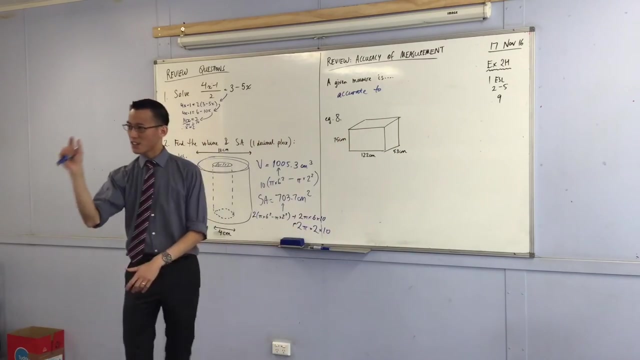 When you're talking about this idea of accuracy right, the phrase I want you to remember is that a given measure is accurate to Okay. now, if I have, for example, if I have, a mid rule right and it's got one centimetre blocks, what would you say is the accuracy? 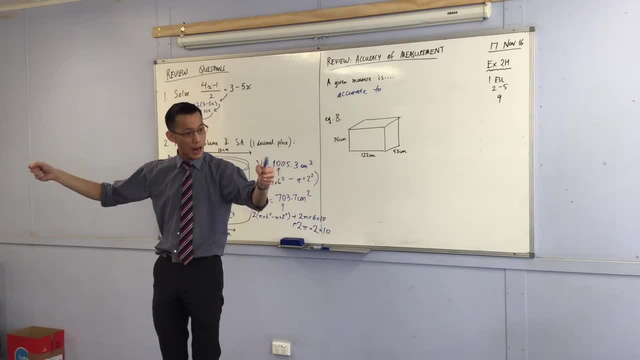 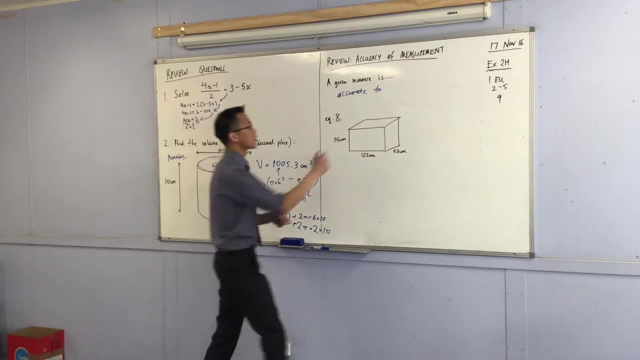 of that metre rule You'd go a half a centimetre right, because if you're measuring something and it's not quite on the dot you can generally say it's closer to one or the other right. So we would say it's accurate to plus or minus a half of the smallest division, which in 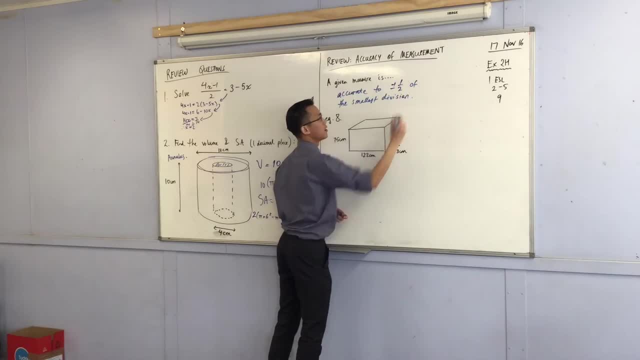 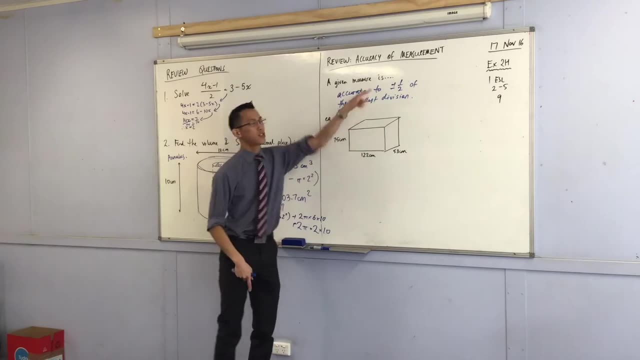 the case I just mentioned was a centimetre. Okay, if you've got something which is measuring to the metre or to the foot or whatever, then you're going to get plus or minus a half of a metre or a foot or whatever It could be. 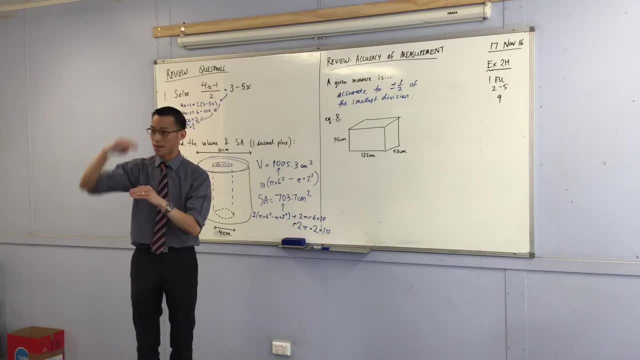 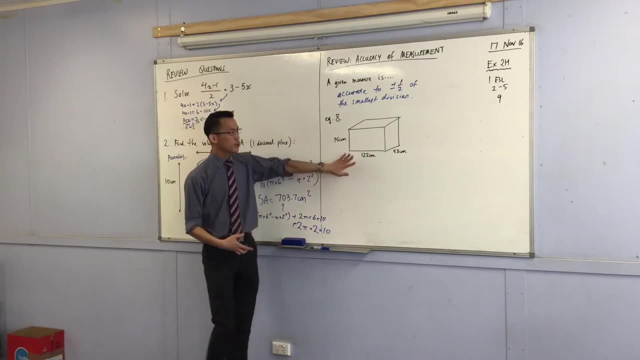 degrees like rotation. it could be degrees on a thermometer, whatever unit that happens to be. you're just looking for the smallest division. Now, what's nice about this is that when you look at something like this, maybe you want to just jot this down. okay, this is actually question 8 from the exercise you're about. 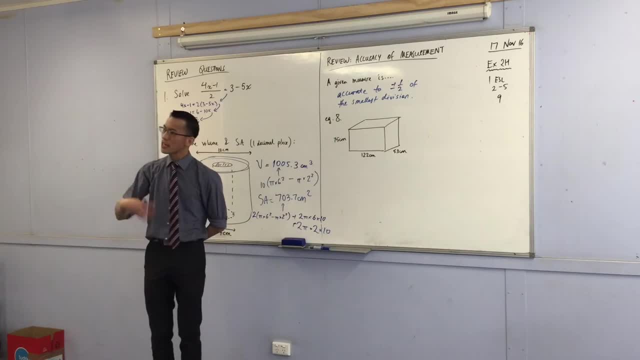 to start, which is why I haven't assigned question 8.. You can know, even without saying it, that you're going to get a plus or minus a half of a centimetre. So if you're seeing the measuring instrument, you can know what the level of accuracy was. 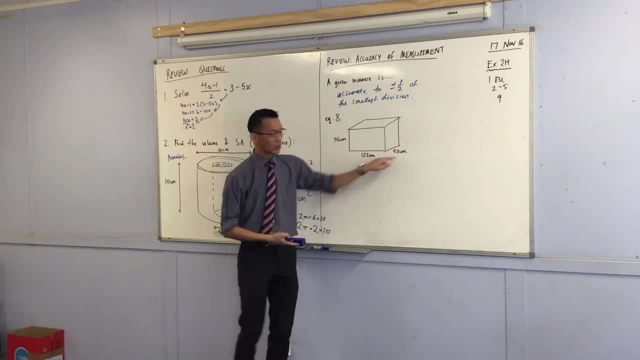 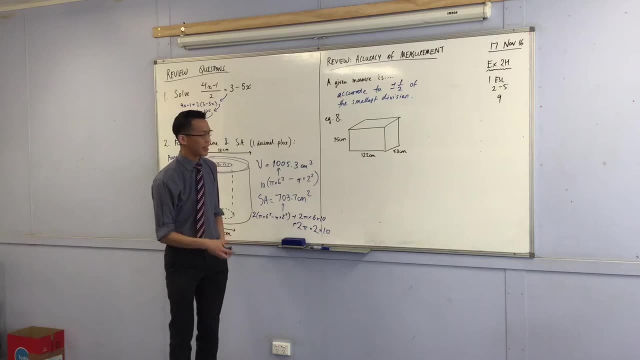 by looking at the measurements that have been provided to you. okay. So when you look at these, what was used to measure this? What was the accuracy for it? It's going to be by the centimetre right. It clearly can't be like the metre something. 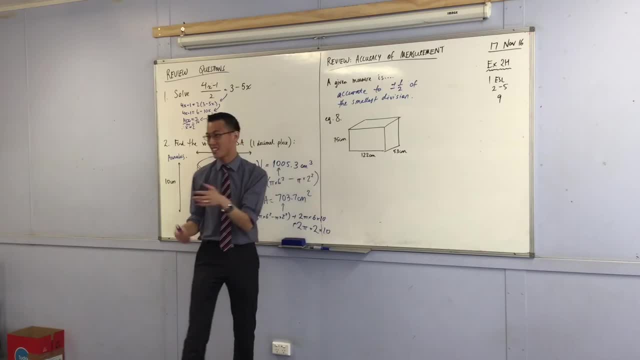 like that. this would be too inaccurate to do this, and if they had it to the millimetre, you'd have some decimal points going up there, so that's fine. So, for starters, let's work out What is the volume of this solder. 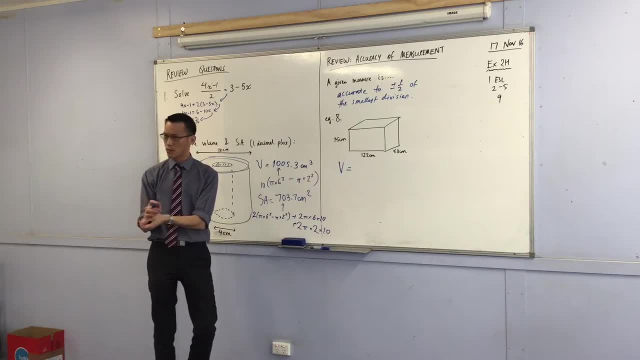 Just as measured. okay, it's a nice easy rectangular prism. so what am I going to do with these numbers? 1,, 2,, 3,, 4,, 5,, 6,, 7,, 8,, 9,, 10,, 11,, 12,, 13,, 14,, 15,, 16,, 17,, 18,, 19,, 20,, 21,, 22,, 23,, 24,. 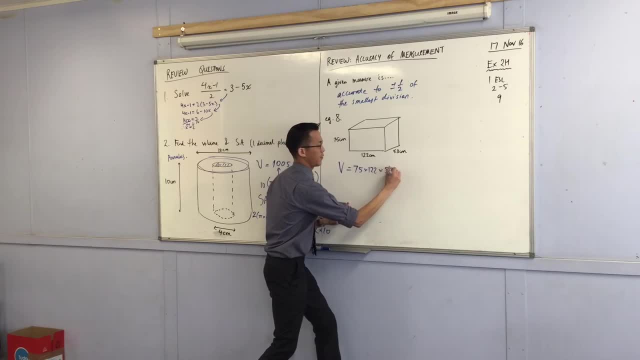 50.. Yeah, I'm just going to multiply them all together, aren't I? So I'm going to go 75, 122,, 53.. Okay, can I have a number Anyone? Four, eight, four, nine, five, oh, 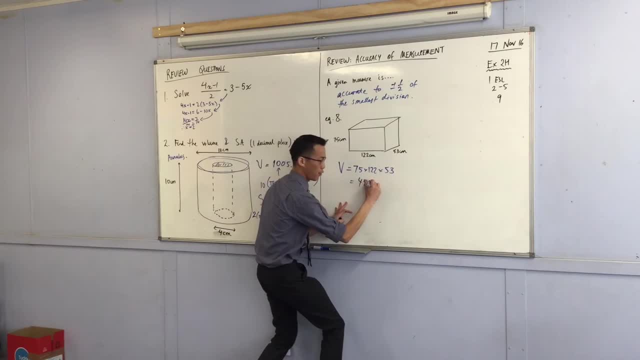 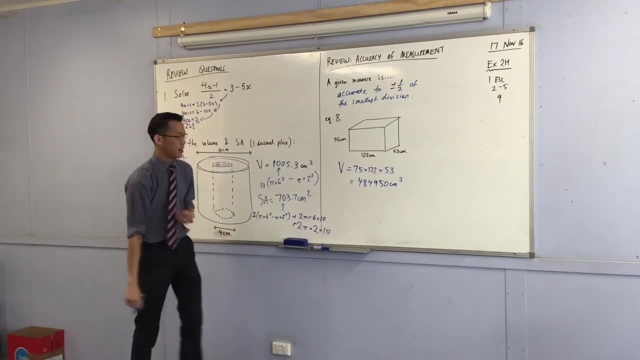 Four, eight, four, nine, Yeah, five oh, Five oh, And that's cubic centimetres. Yeah, pretty big number, but that's because these are pretty big numbers and we're multiplying them together, so that's fine, okay. 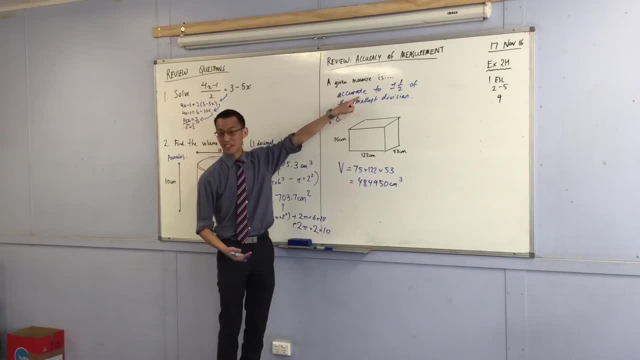 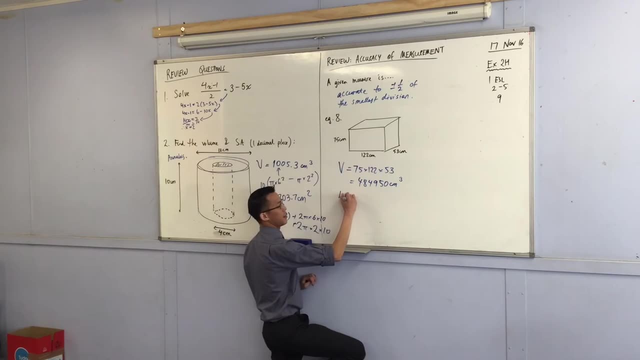 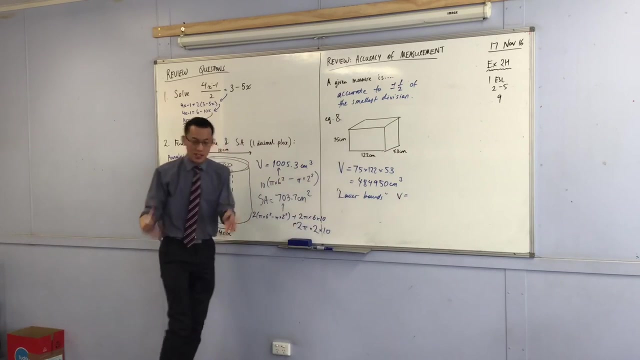 Now we know, though, that, because it's not necessarily perfectly accurate, the real volume might be smaller, or it might be bigger, okay, So what we're going to do is we're going to take the lower bound, Okay, and we're going to work out the volume based on if these were actually not the 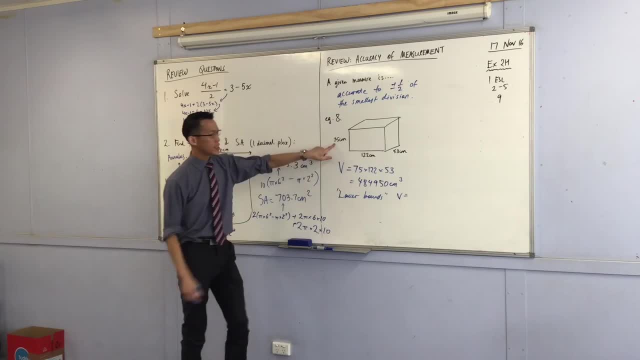 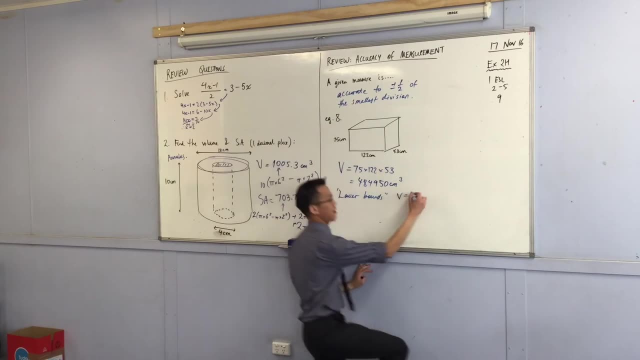 exact. but like what if they were smaller than that? right. so this one over here, 75- the smallest it could possibly be if it's half a unit, is going to be 74.5, right. in exactly the same way, the 122 could have been 121.5. and the last one, 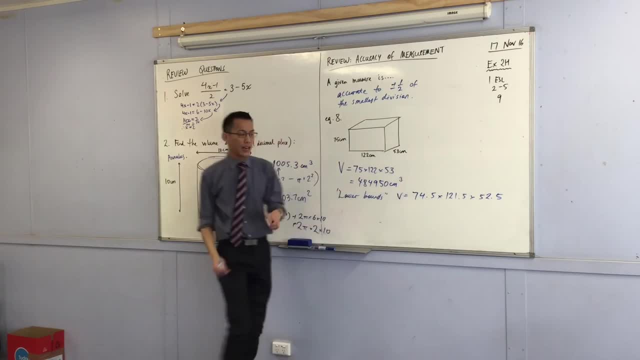 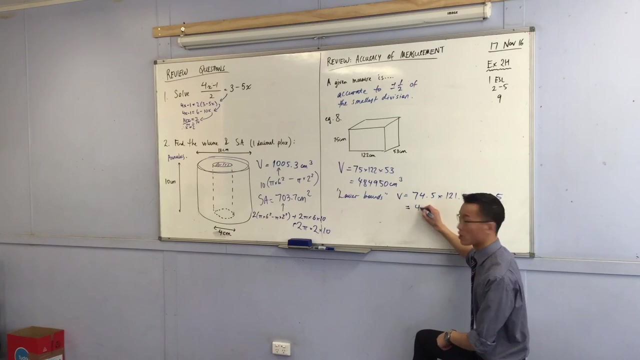 could have been 52.5. okay, so it's only half a centimeter difference. what kind of um, what kind of difference will it result in the volume? well, again you turn to your calculator and we're going to get something with decimal places, aren't we? what do we got four, seven, sorry, two, one, six. okay, now let's have a look how. 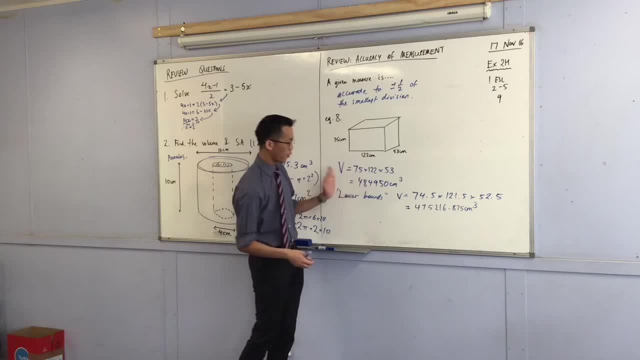 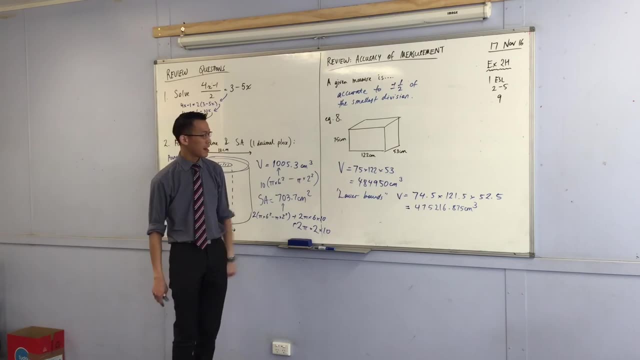